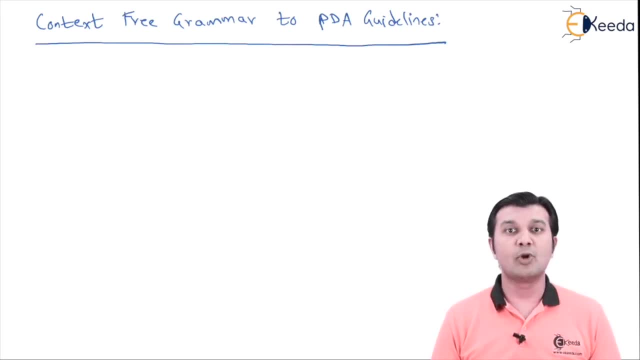 form Unless, and until it is in GNF, you will not be able to do anything to get it converted to Pushdown Automata. So, friends, let us discuss the steps as well as the problem in the same video. So over here we say: given context-free grammar G equal to VTPS, we are going to define a. 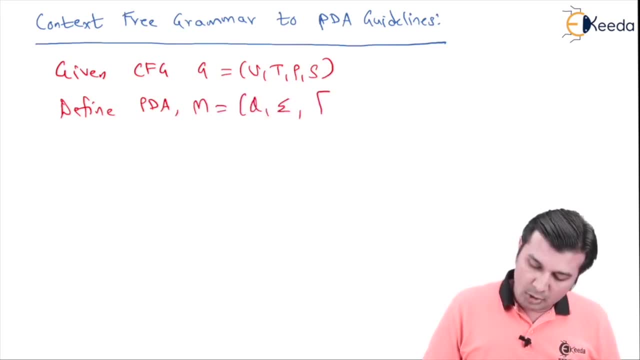 GRIBAC normal form, which is mathematically represented as M equal to Q, summation G del Q0, Z0, F. Next, I say first and foremost thing: we are going to express the CFG in the GRIBAC normal form, which says all the production should be of the form. X gives A alpha where 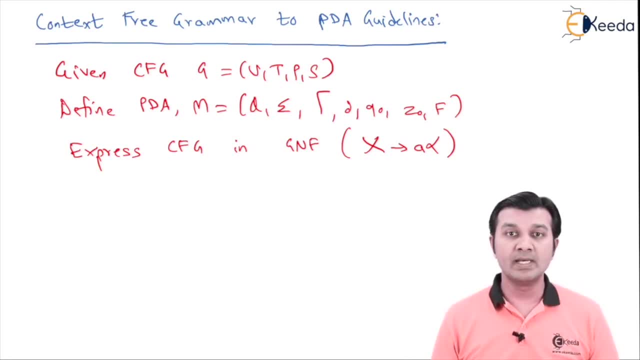 A is going to be a terminal And alpha is going to be in sentential form, that is, any combination of variables or terminals. The next is: I say over here, my Q is going to be my Q0 always. Then my next thing: summation. 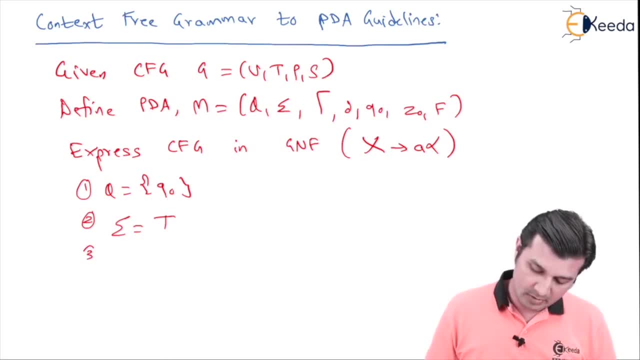 is going to be the T in the context-free grammar. Third one: my G is going to be is equal to my set of G. So I said it is going to be set of variables which I call by V dash. Fourth one: my Q0 is: 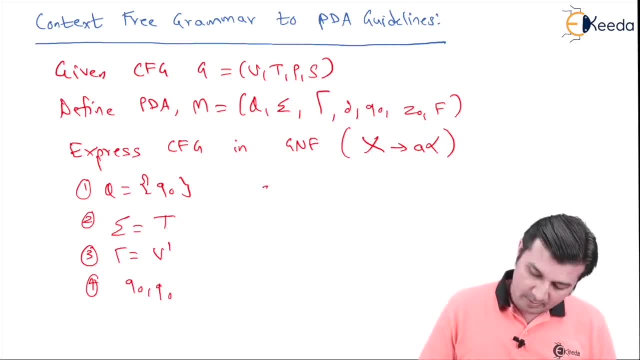 going to be is equal to Q0. again My fifth one: Z0 is going to become the start symbol of the context-free grammar. Sixth, one final state is not going to be present over here Why that will understand when I start with the problem. 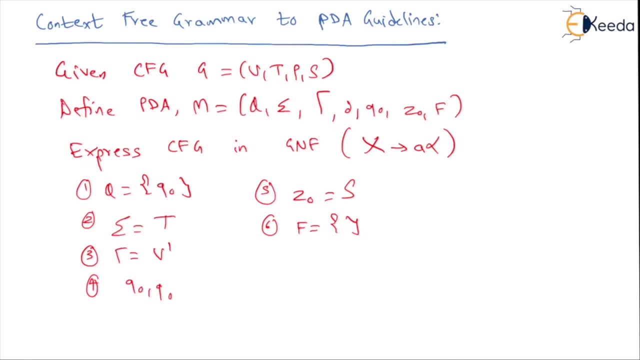 10. An important thing. we have simply two rules for convergence. So let me write down the rules over here. So the first is my rule. one is: if I have a production movie of the form a gives small a, b, c, first and foremost thing, it is in CLF and how do you convert it to PDA? 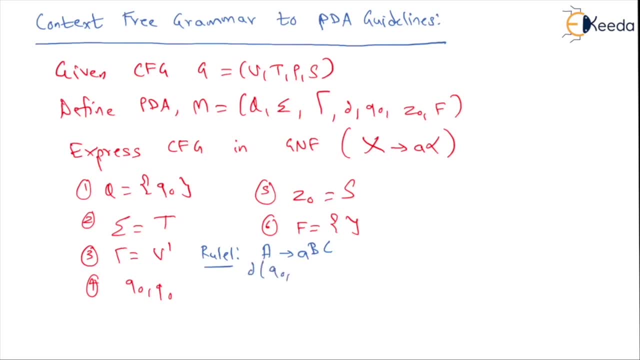 You simply say del q0 on small a. when the stack top is capital, A goes to q0 and stack happens to be converted to b, c. Similarly my rule two. it says: for a production of the form a gives a, you write del q0 on a, b, c. 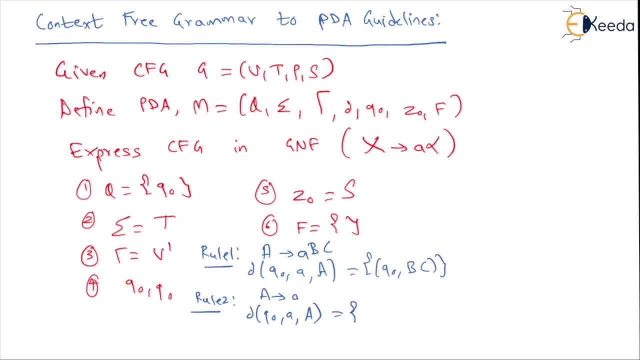 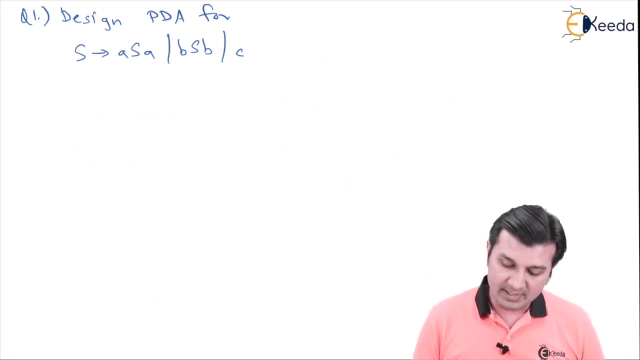 When the stack top is a, goes to q0 and performs a pop operation. Simple as that. Just remember these two rules and the problem is solved. So now let's start with the problem and try to get a deeper understanding of the same. So, friends, the problem which is given to us says: design a push down automata for the following: 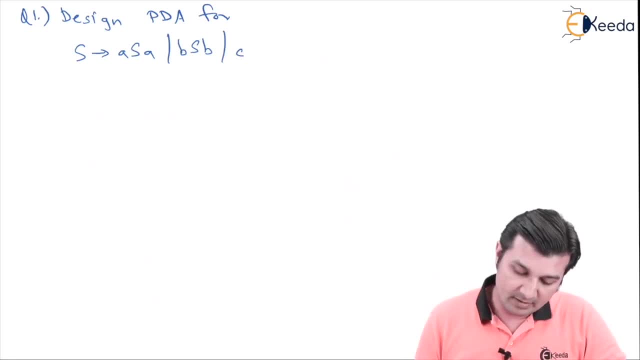 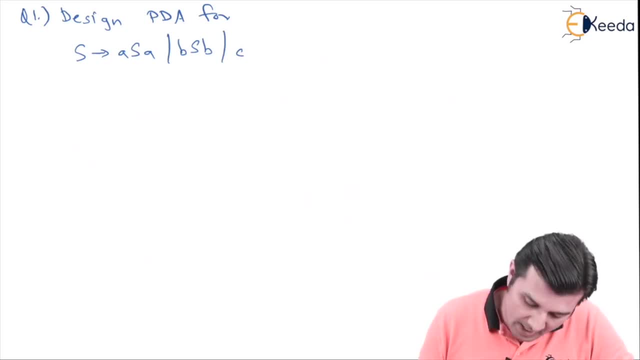 First thing is we have to get it converted to g and f and therefore I say in the solution: let my c1 be deriving small a and c2 be deriving small p, which makes my s converted to a, s and b. Yes, I know, the question over here is: why have we not replaced for first small a? also because we want it in the form of reback, normal form. 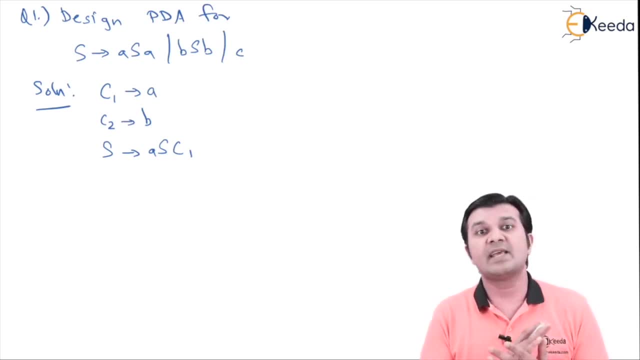 We are keeping the first terminal as it is and rest everything. we are getting it converted to alpha with the help of c1 and c2 respectively. Therefore, I now say again: keep b as it is, s, followed by c1. And the last one is going to be c as it is. 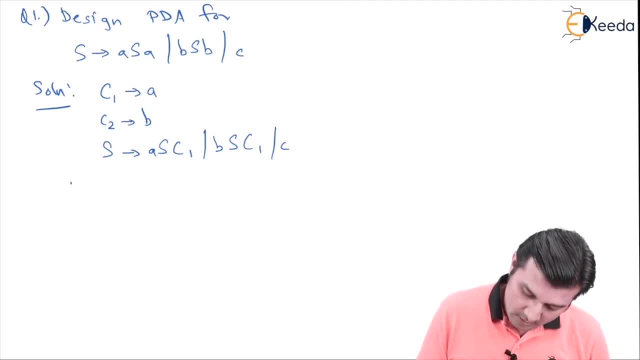 Further going ahead over here, I have my q to be my q0.. Next, I have my input alphabet as a, b and c respectively. Next, I have my input alphabet as a, b and c respectively. Third, my stack symbol g as the same, that is, a b. 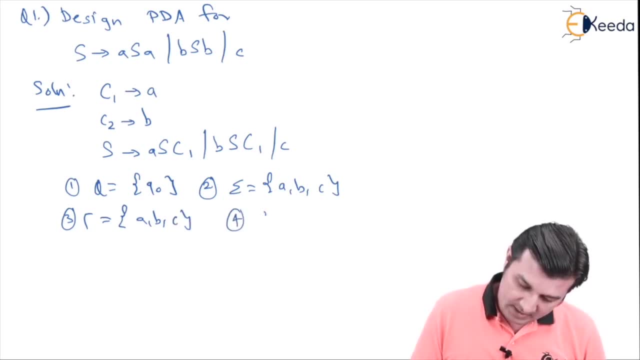 and C respectively. My start state q0 remains as q0 always. My z0 is going to be the start symbol, which is capital S, and, as I told you before that the final state is going to be empty. Let's go ahead and solve the problem now. Before solving the problem, let me rewrite the rules for. 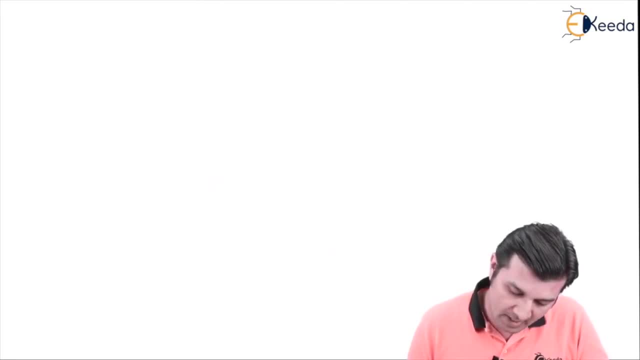 this problem. So we have the rules over here. Let me write it: a gives a b c, We say del q0 a a equal to q0 b c, And for a gives small a, I say del q0 a. a performs the pop operation q0 epsilon, without changing the state. 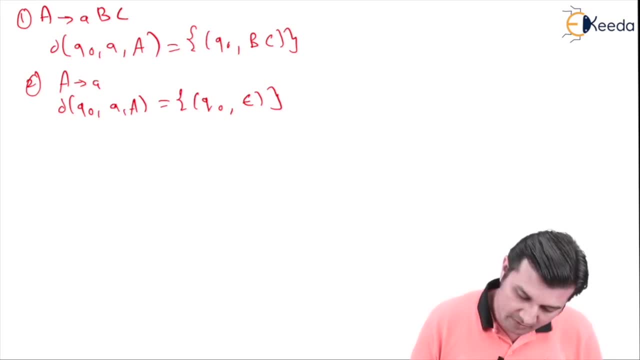 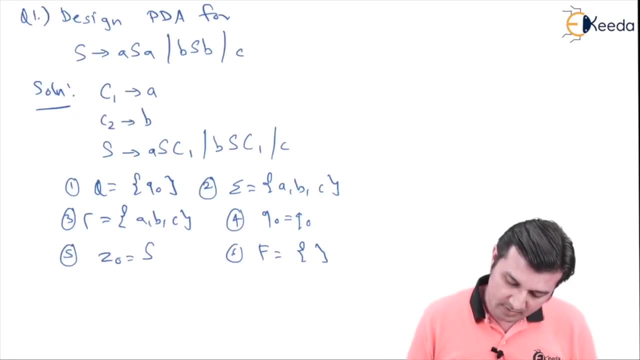 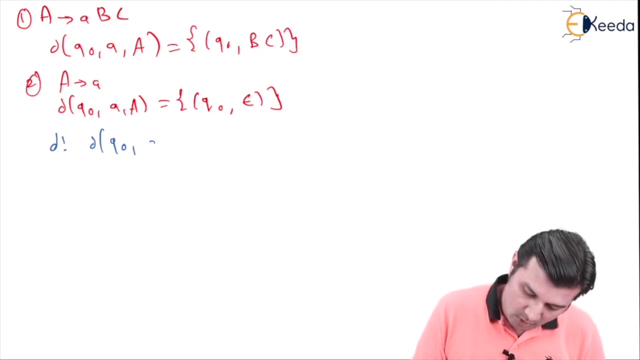 Let's start with the problem. Now for the first production we have. I am talking of this one: sqasc1.. Del q0 on a, when the structure goes to a toостоck, is엦 goes to q0, and I have sc1 on the stack. 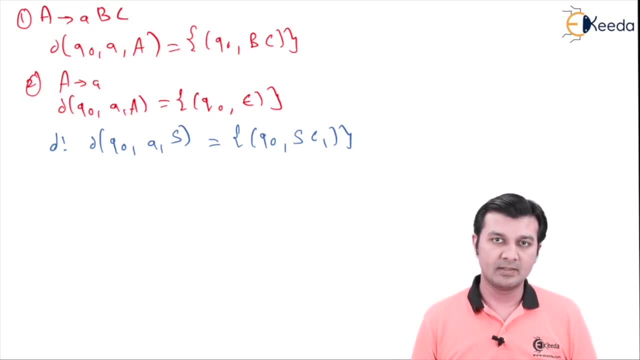 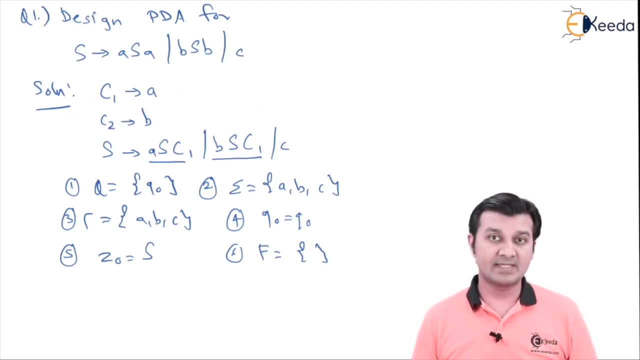 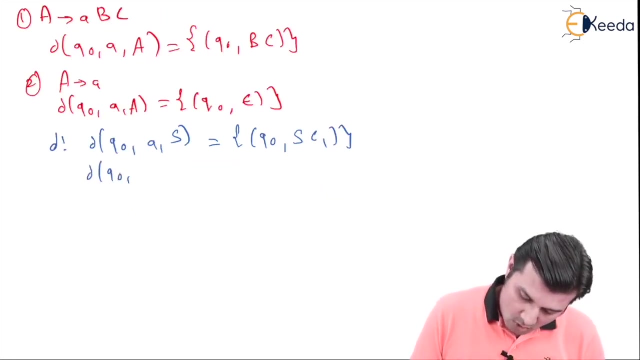 s goes to q0 and I have sc1 on the stack. Next for the second production, which is this: s gives b, sc1.. Again, using rule 1, I say q0 on b when the start solve is s- 👉. s goes to q0 and I have s- desktop here. 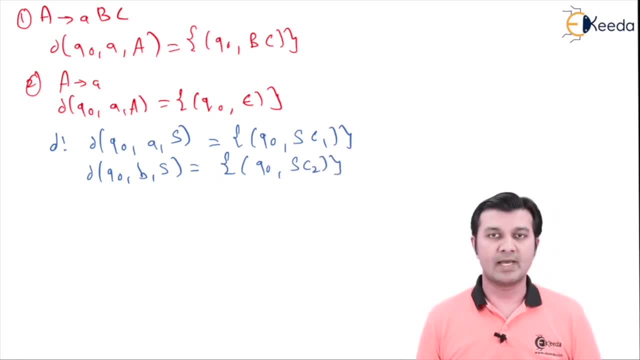 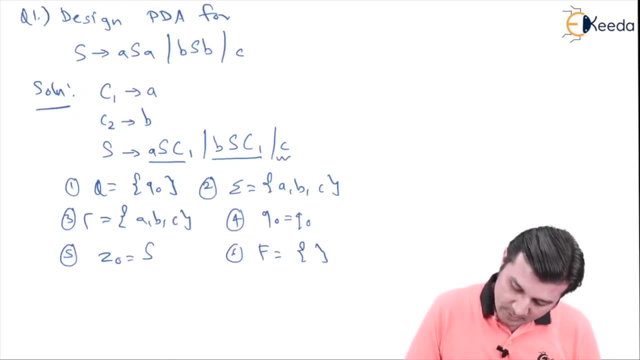 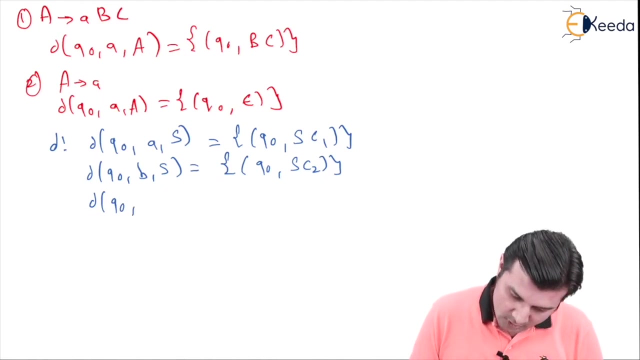 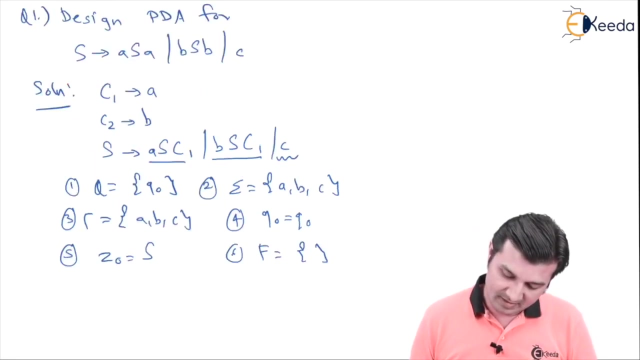 what I did mean is I will write this down: the first production has the first addition of s as q0.. C2 on the stack. Going ahead for the third production, which is simply the C, using rule 2, I say Q0 on C, when the stack top is S goes to Q0, comma epsilon. Next one for C1 gives. 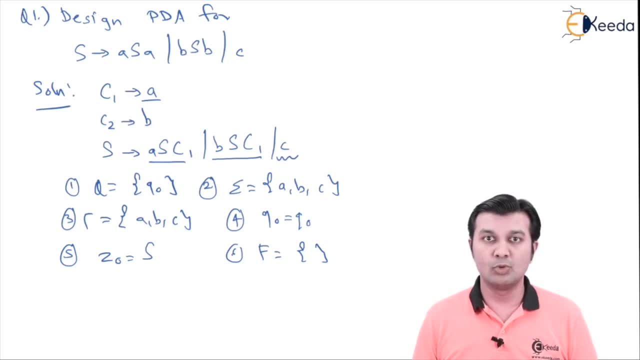 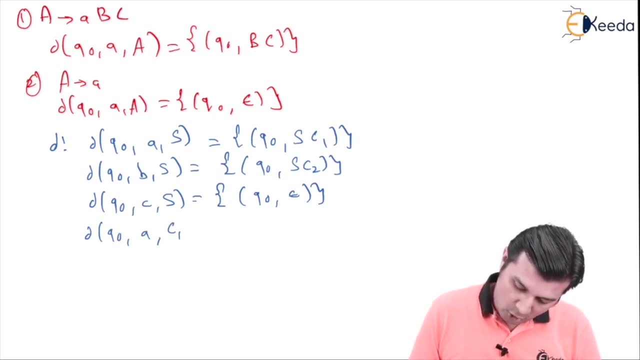 A, this production, I say using rule 2,- Q0 on A, When the stack top is capital, C1, goes to Q0, comma, epsilon, by performing the pop operation. Lastly, Q0 on B, when the stack top is C2, again goes to Q0,, performs the pop operation. and 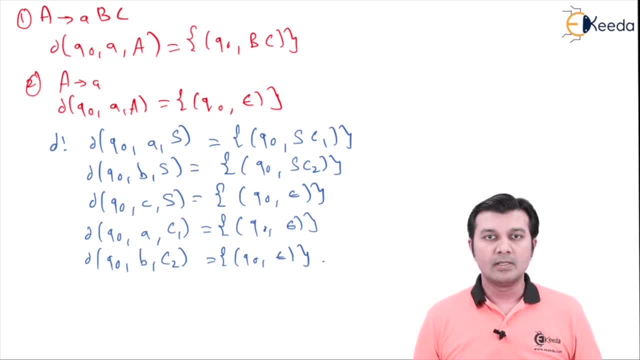 here we stop. There are definitely going to be a lot of questions in your mind As to how this thing is actually going to work. So here comes an example for you to verify whether the machine is working fine. So maybe I say example, I will state Q0 input. 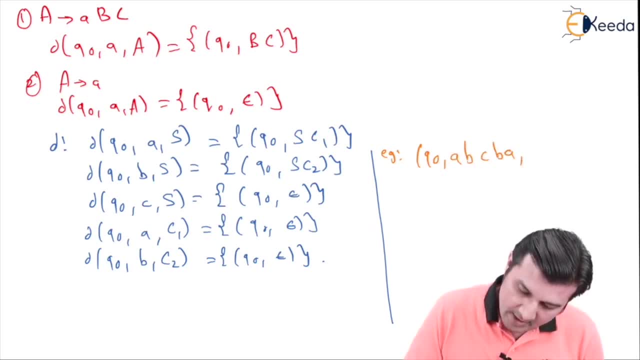 is A, B, C, B, A and stack top is S. So Q0 on A when the stack top is S goes to Q0 comma epsilon. let me label the numbers 1,, 2,, 3,, 4 and 5.. So Q0 on A when the stack top is: 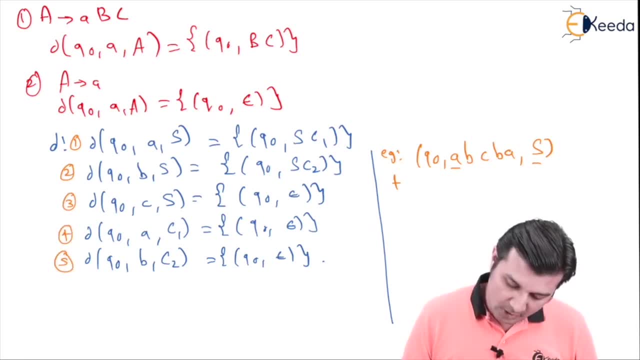 S using rule 1, I say: go to Q0, what remains is B C, B A, and we say: we are going to push over this. S becomes S C1.. S becomes S C1.. We are going to push over this. so S becomes. 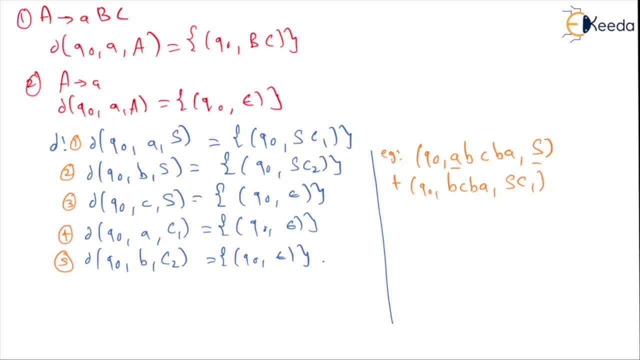 S C1.. S becomes S C1.. S becomes S C1.. We are going to push this over. S becomes S C1. And this and this working with context, free grammar. So what we are showing over here is what is pushed. 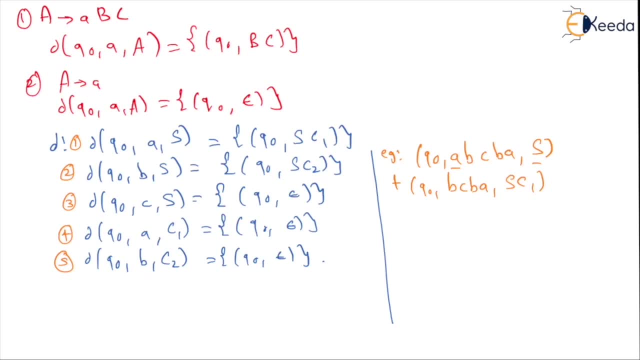 in place of water. So the representation over here is going to be slightly different from what we are studying till now in all the previous problems. Further: Q0 on D when the stack top is S. Q0 on D when the stack top is S using rule. 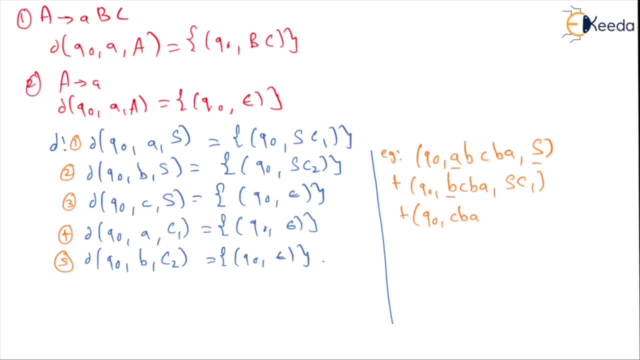 2, I say: go to Q0,. what you have is CBA and we have S, C2, C1 over here. Further going ahead, Q0 on C when the stack top is S, using rule 3, I go to Q0,. BA remains over here and 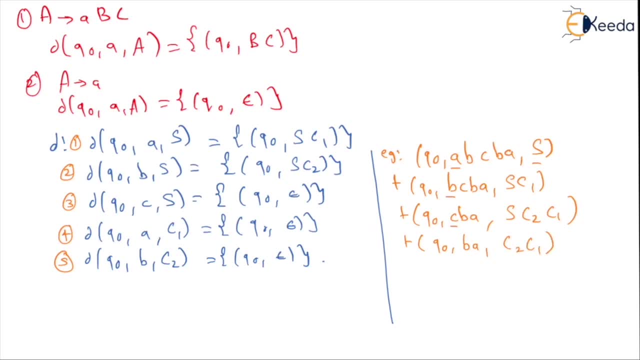 since I pop out the S, I have C2 and C1. Then Q0 on D, when the stack top is C2, using rule 5, I go to Q0, I have A pending and C2 is popped and therefore only C1 remains on the stack. 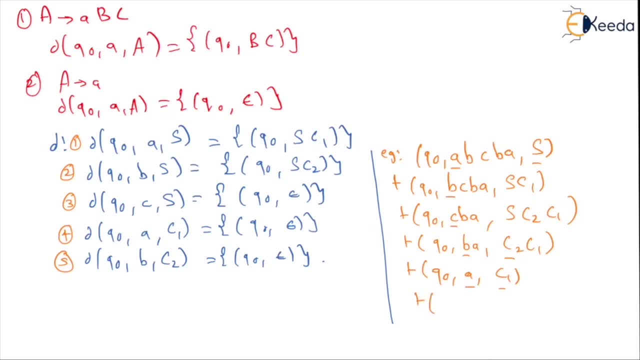 And lastly, Q0 on A. when the stack top is C1, using rule 4, I go to Q0, epsilon remains over here and epsilon remains over on to the stack. Since both of them contribute 0, I go to Q0, when the stack top is C1, I go to Q0, then. 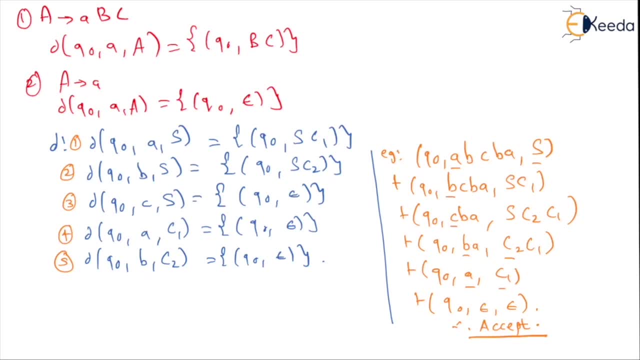 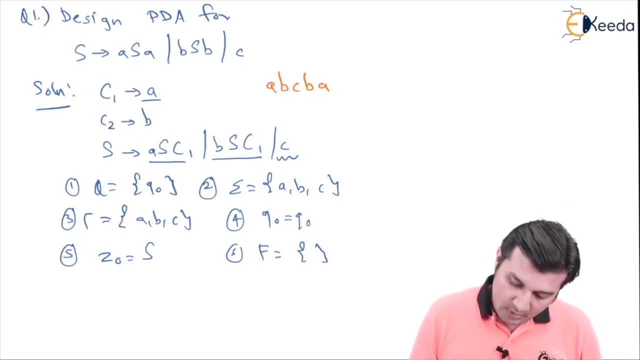 to epsilon. at the end I say this input will be accepted by my push down automata. If you verify this particular input- A B, C, D A- it's a problem. A B C D A. We can see that. 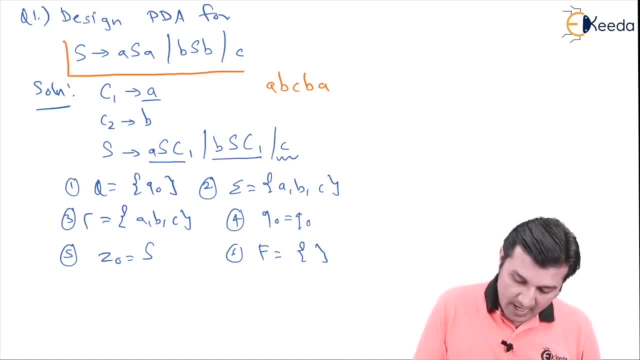 this particular input will also be accepted by this context-free grammar. You can work on with LMD and RMD, as we tried in the previous video and see that this particular string is very well accepted by my context-free grammar, as well as the equivalently designed push down automata. 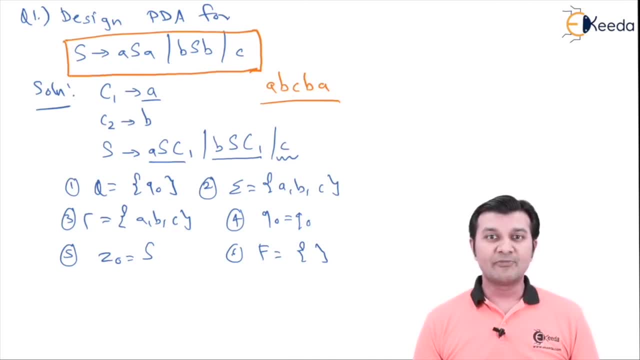 So, friends, with this we complete the full chapter on push down automata. I am very sure every one of you might have understood the minute details of this chapter. See you in the next session, where we are going to start with a totally new chapter called as. 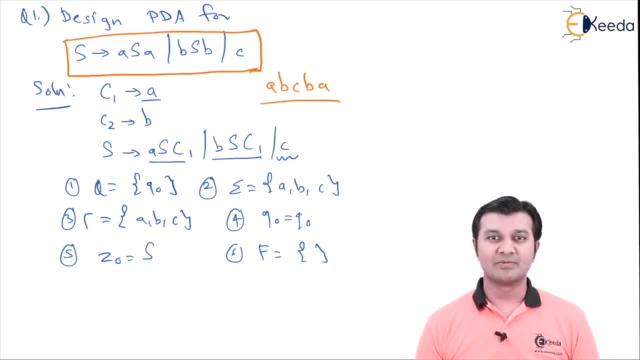 Turing Mushroom. See you, friends. Thank you.